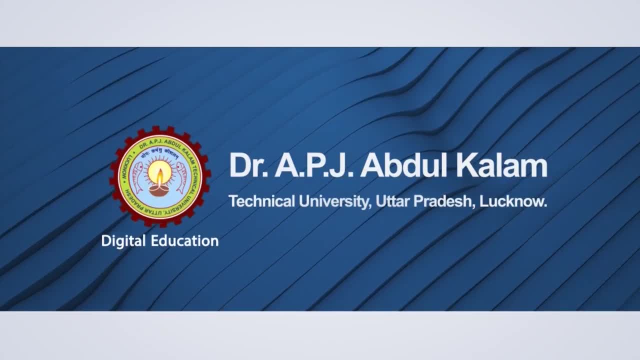 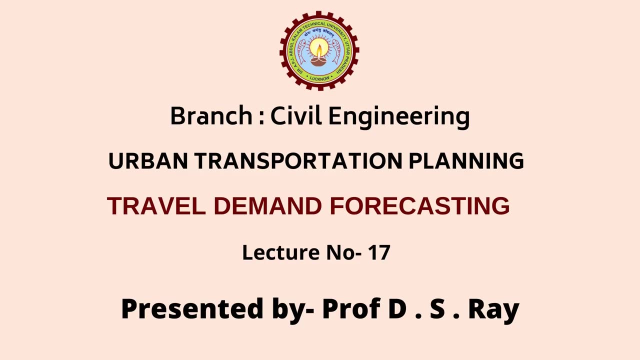 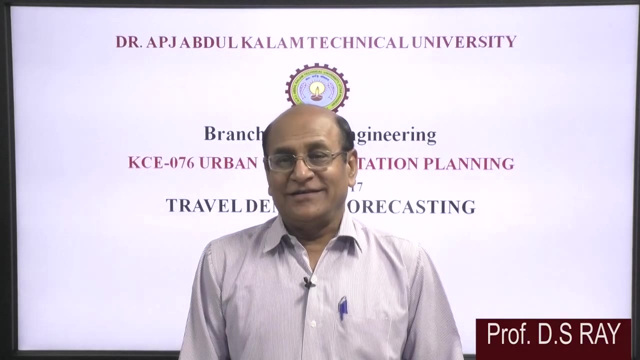 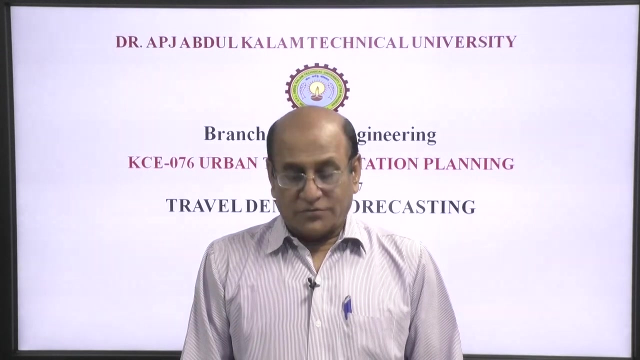 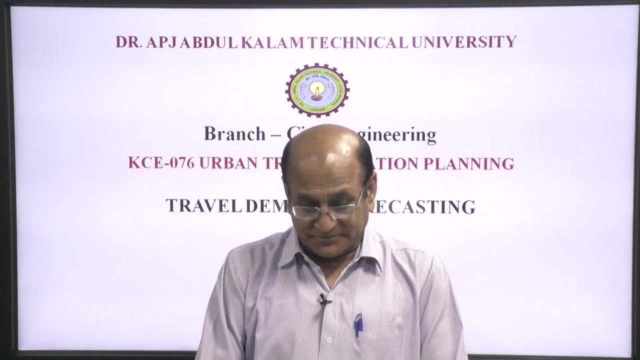 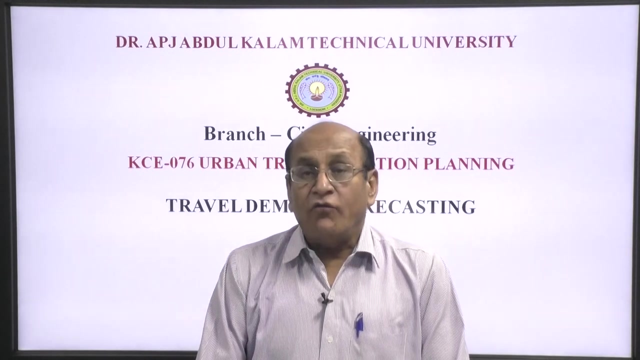 Welcome class Myself, Professor D S Rai, Professor Department of Civil Engineering, BBDA ITM Lucknow. Today we will take up course KCE 076, Urban Transportation Planning, in which today we will take up lecture 17, Travel Demand Forecasting. References that: 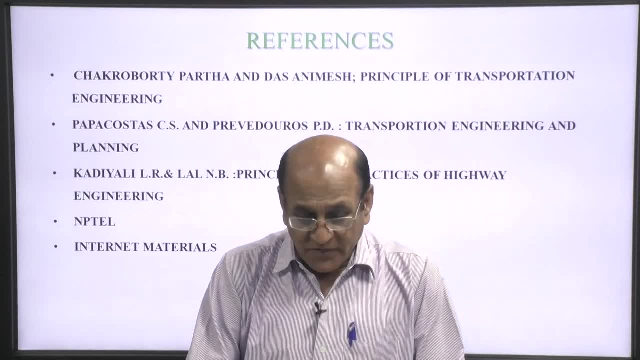 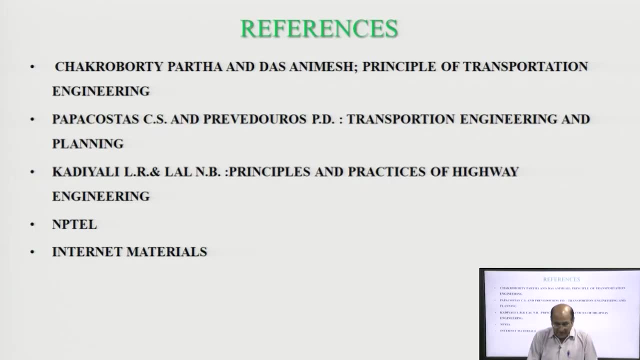 I have taken Chakravarthy, Partha and Das Animesh, Principal of Transportation Engineering, Pappacosta and Pravidandas, Transportation Engineering and Planning, Kadiali and Lal Principal of Principal and Practices of Highway Engineering. Some material have been taken from NAPTR and some material have been taken. 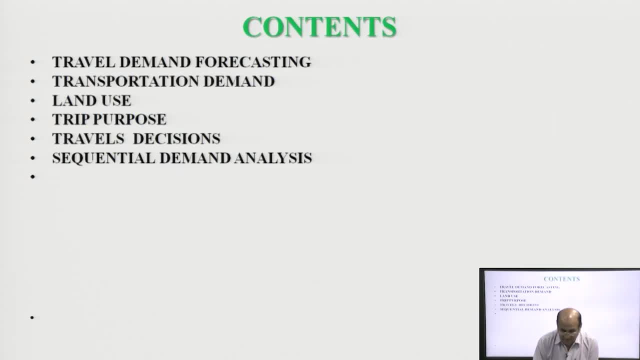 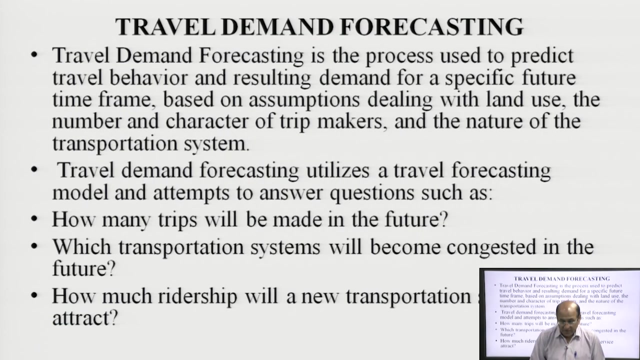 from internet The contents. today we will take up Travel Demand Forecasting, Transportation Demand, Land Use, Trip Purpose, Travel Decisions, Sequential Demands Analysis. So first of all we will take up Travel Demand Forecasting. Travel demand forecasting is the process used to predict travel behavior and resulting demand. 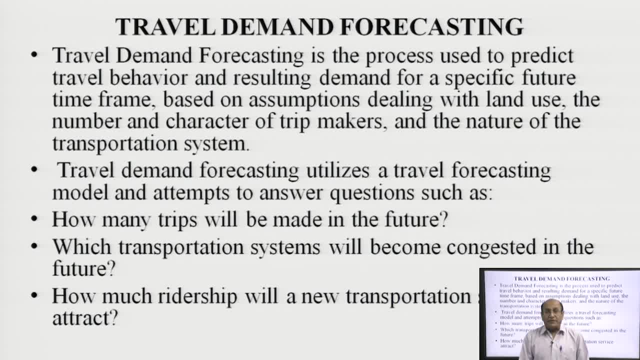 for a specific future time frame based on assumption dealing with land use, the number and the character of trip maker and the nature of transportation system. Travel demand forecasting utilizes a travel forecasting model and attempt to answer questions such as how many trips will be made in future? which transportation system will become congested? 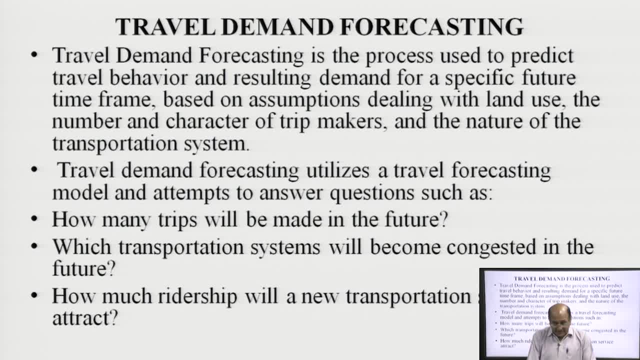 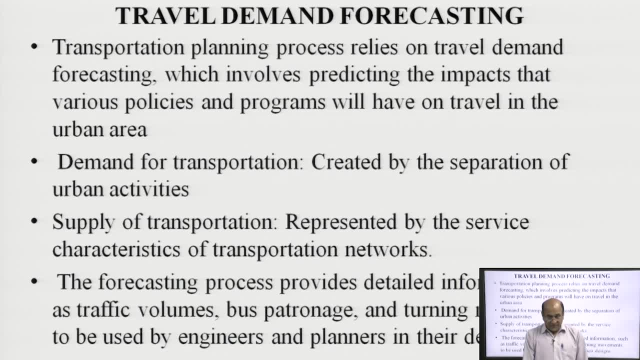 in future? How much ridership will a new transportation service attract? Transportation planning process relies on travel demand forecasting, which involves predicting the impact that the various policies and program will have on travel In the urban areas. the demand for transportation created by the separation of urban activities. 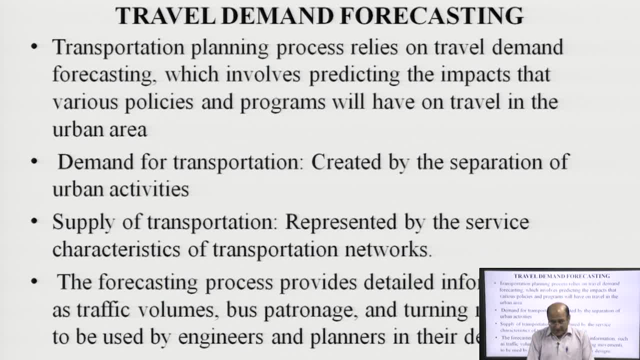 Supply of transportation, represented by service. characteristic of transportation and network. The forecast process provide detailed information, such as a traffic volume, bus passenger and passenger. The transportation process provides detailed information, such as a traffic volume, bus, passenger and passenger. It also provides detailed information such as a daily route cost우�ر지오. 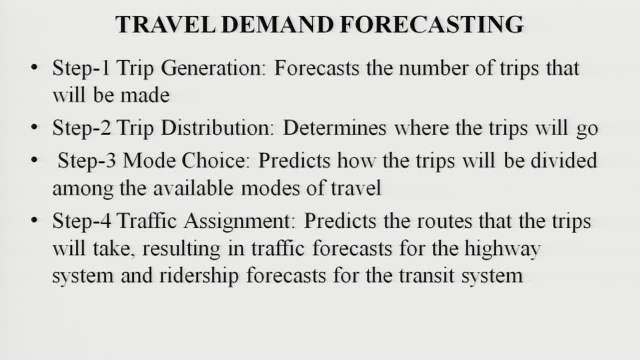 To be used by the engineers and planning of their designs: Travel demand forecasting. We will take up different steps in a Step 1 trip Generation forecasts the number of trips that will be made. Ninety-one trips aged fifty-two are provided as of next universities like Indianapolis. 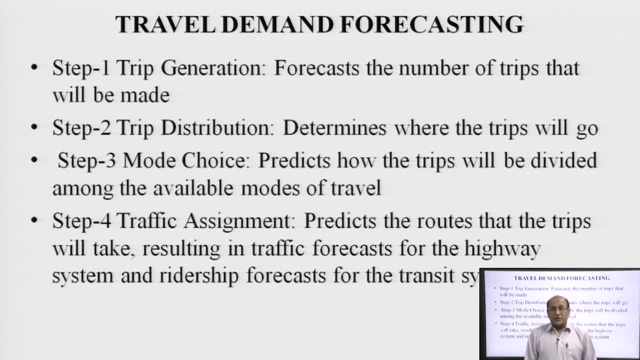 Limited to jobs have been dispensed Two. So DSG during international And andeling, we will introduce changes. it will improve the transportation size, falling 4 times much. Trip distribution: determine whether the trip will go. Step 3, mode choice: predict how the trip will be divided among the available mode of travel. 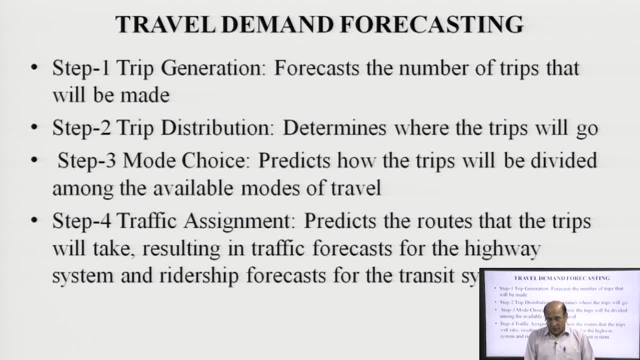 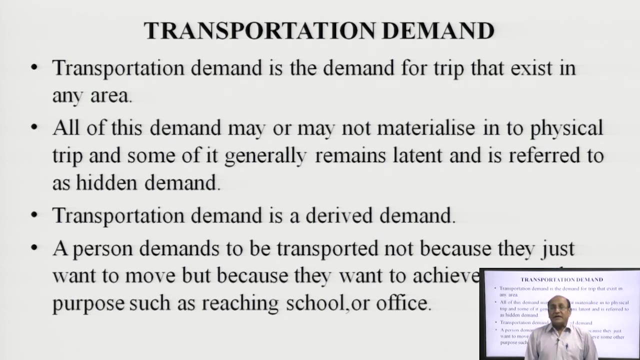 Step 4, traffic assignment predict the route that the trip will take, resulting in traffic forecast for the highway system and ridership forecast for the transit system. Transportation demand is the demand for trip that exist in any area. All of the demands may or may not materialize into the physical trip. 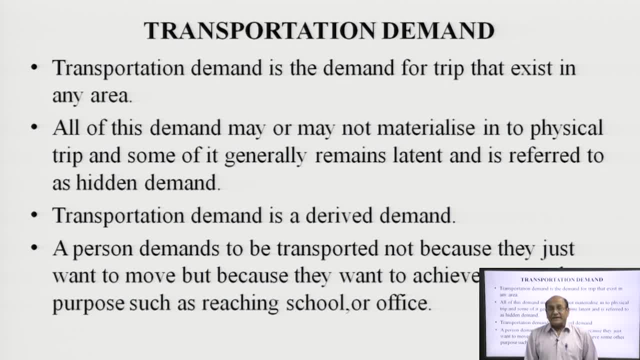 And some of it generally remains latent and is referred to, referred as hidden demand. Transportation demand is a drive demand. It is very important Because trips are very important. Transportation demand is usually not made for the itself means no one can wander on the roads. 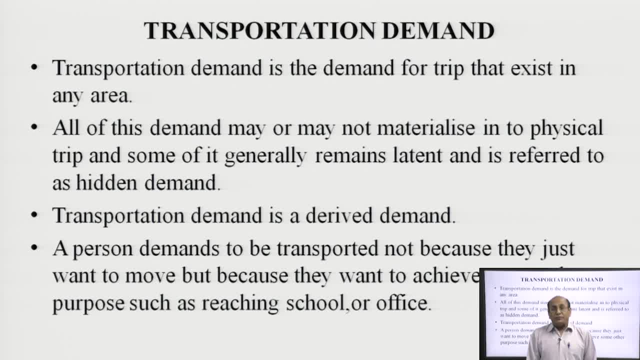 But we have to go for school, then a trip will come in existence. When we will go for the market, then the trip will come in existence. So in this way, transportation demand is a drive demand. So in this way, transportation demand is a drive demand. 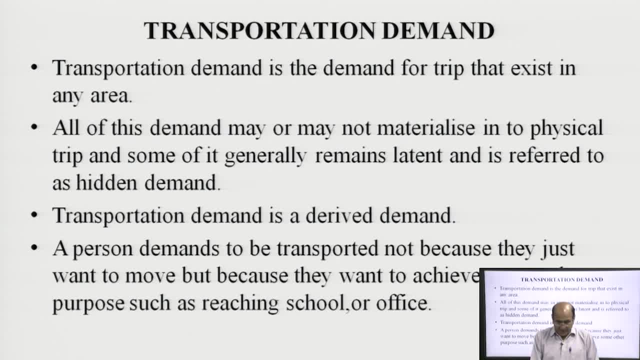 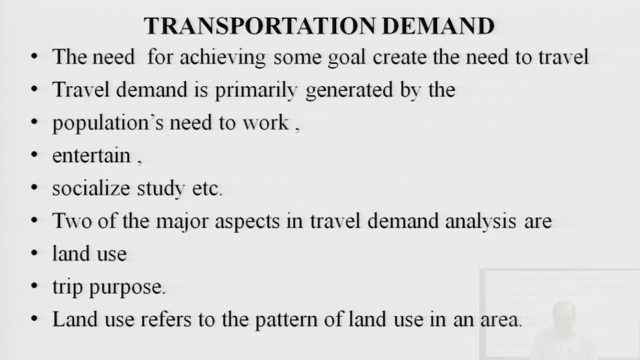 So in this way, transportation demand is a drive demand. A person demand to be imported, a person demand to be transported, not because they just want to move, but because they want to achieve some other purpose, such as reaching a school, etc. The need for achieving some goal create the need to travel. travel demand is primarily 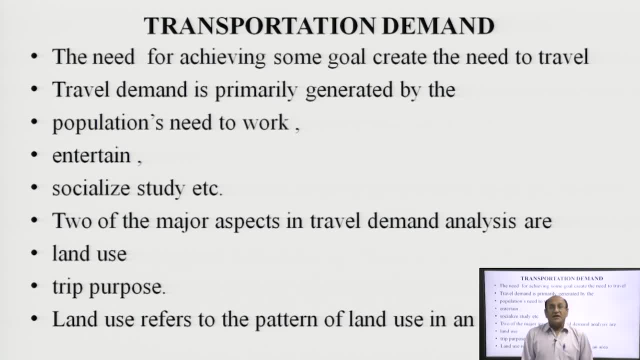 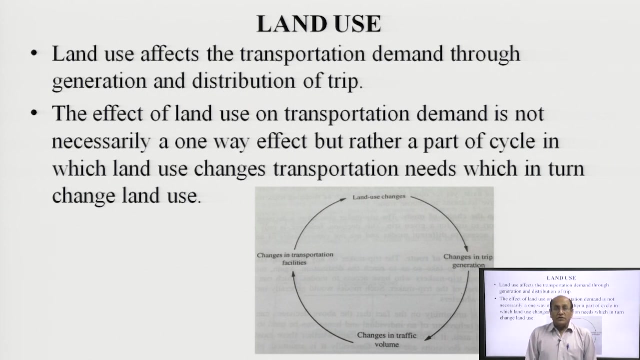 generated by the population: need to work, entertain, socialize, study, etc. Two of the major aspect in travel demand analysis are land use, Trip purpose. the land use referred to the pattern of land use in the urban areas. Land use affect the transportation demand through generation and distribution of a trip. 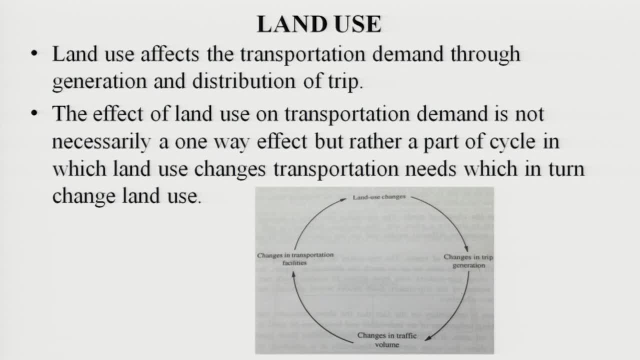 The effect of land use in transportation demand is not necessary A one way effect, but rather a part of cycle in which land use changes transportation needs, which in turn changes land use. We can see in this diagram. we see this is the land use and after this land use, then 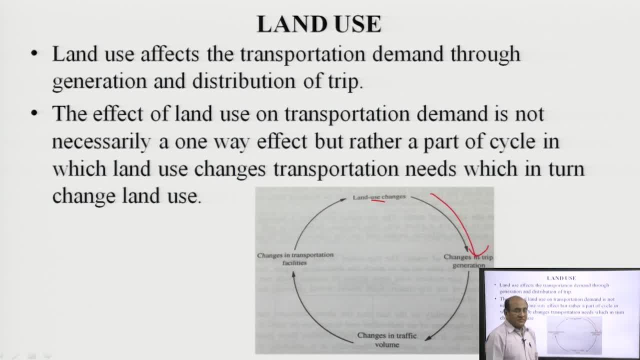 there will be change in the transportation demand, In the trip generation, then this will improve the changes in the traffic volume and after that changing transportation facility. Again this will go for the land use changes means land use changes will make the things every time in a cycle. 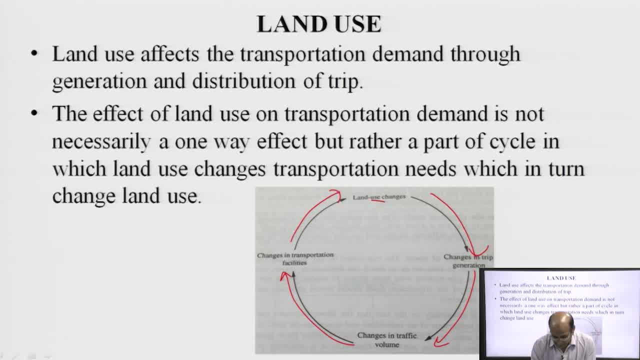 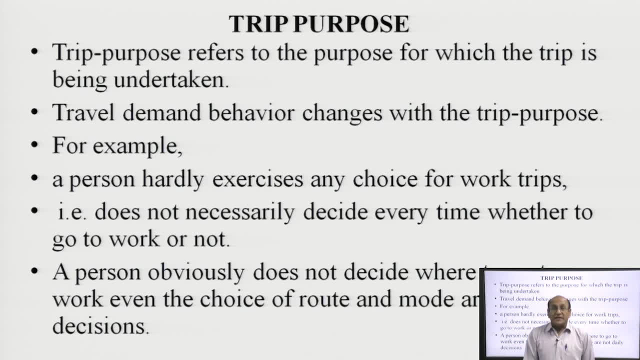 Trip purpose refer to the purpose for which the trip is being undertaken. Travel demand behavior changes with the trip purpose. For example, a person hardly exercise any choice of work trips. that is, does not necessarily determine the travelling responsibility, Even when the person toward the destination is not fully aware whether it is a sociological 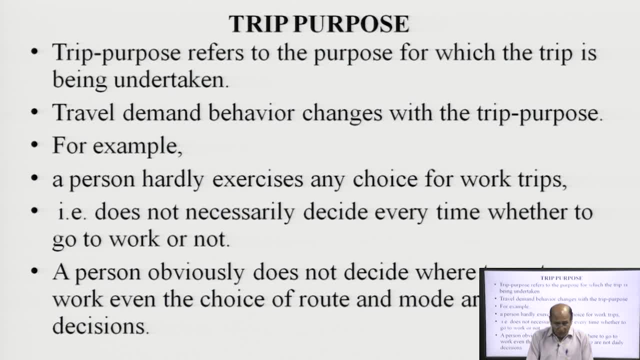 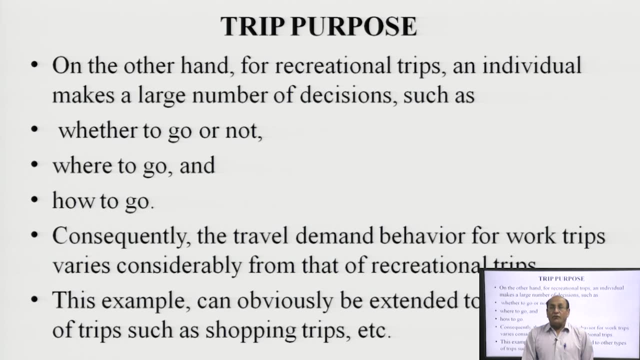 or another social skill related to an activity or other activity. the traveller will decide every time whether to go to work or not. A person obviously does not decide where to go to work. even the choice of route and mode are not daily decision. 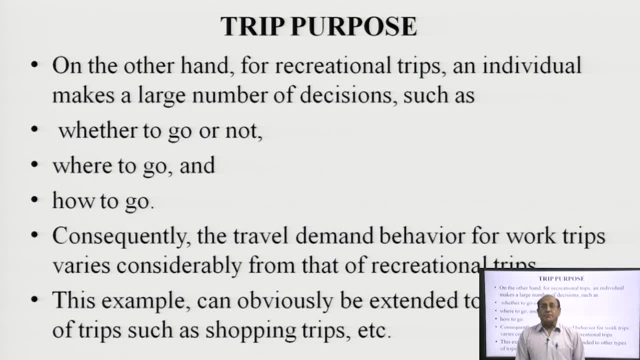 number of decisions such as where, whether to go or not, first, where to go and how to go, this question are asked every time, every persons. consequently, the travel demand we have here for work trips varies considerably from that of recreational trip, the example. 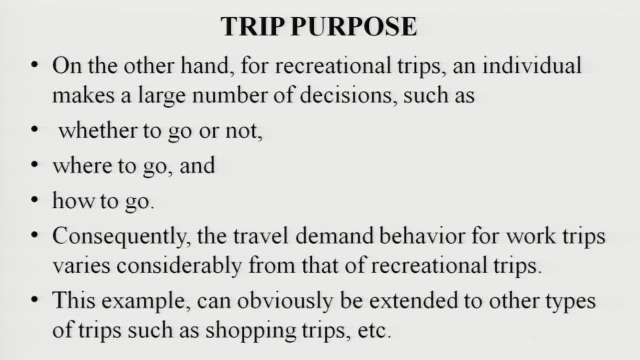 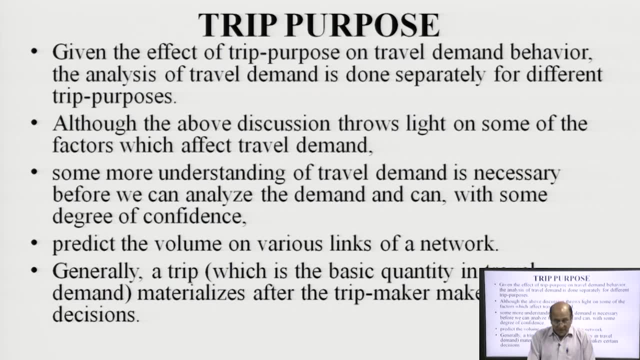 can obviously be extended to other types of trip, such as shopping trips, etcetera, given the effect of trip purpose on a travel demand we have here. the analysis of travel demand is done separately for different trip purposes, Although the above discussion throw light on some of the factor which affect travel. 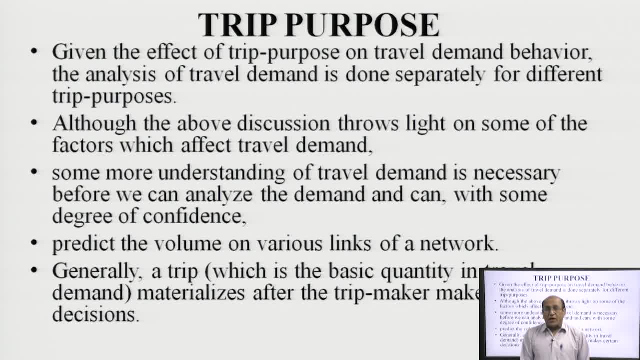 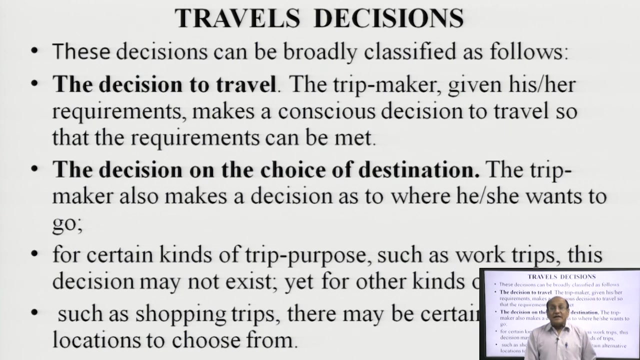 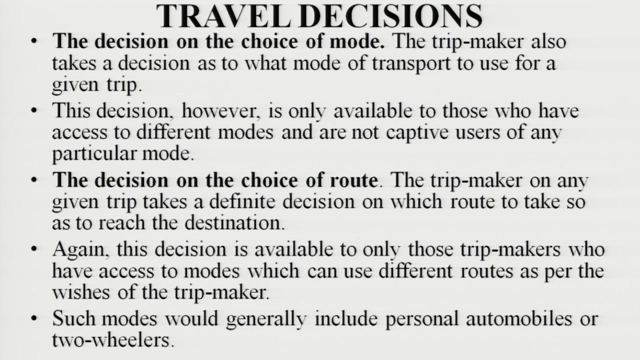 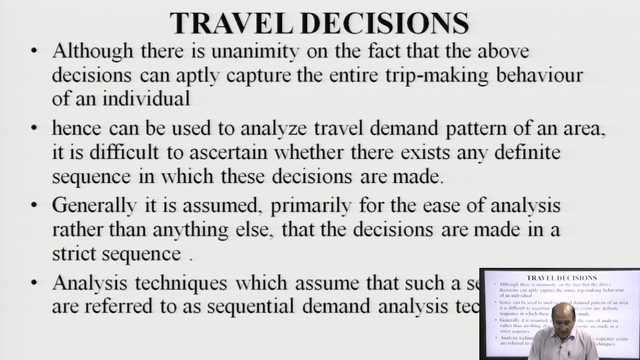 demand. Some more understanding of travel demand is necessary before we can analyze the demand and can with some degree of confidence- There is a unanimities on the fact that the above decision can apply- capture the entire trip making behavior of an individual. Hence he can use to analyze travel demand pattern on an area it is difficult to ascertain. 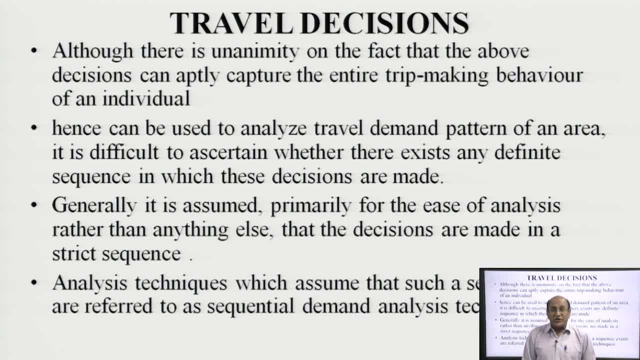 whether there exist and a definite sequence. Generally, it is assumed, primarily for the ease of the analysis rather than anything else, that the decision are made in a strict sequence. analysis techniques which assume that such a sequence exist are referred to a strict sequence. So she is a sequential demand analysis, a technique. 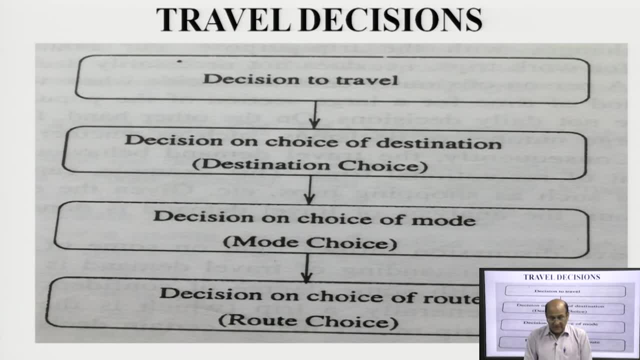 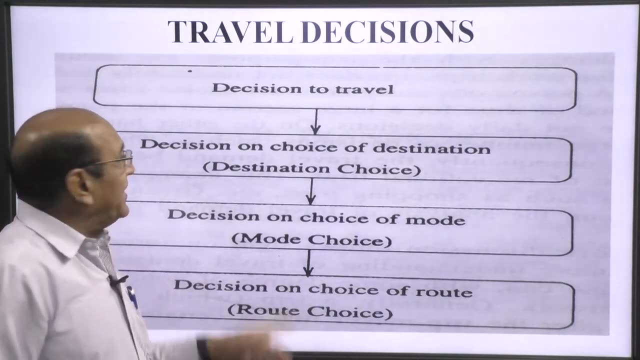 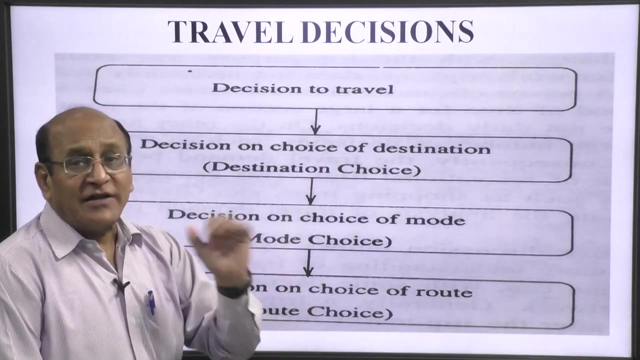 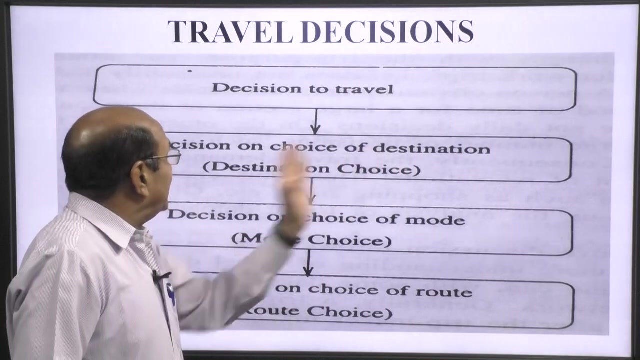 So in this figure we can see a travel decisions. any person can take a decision regarding this one decision to travel. past of all, a person will take a decision whether he has to travel or not. Then, after decision of travel, then decision on choice of destination- which destination? 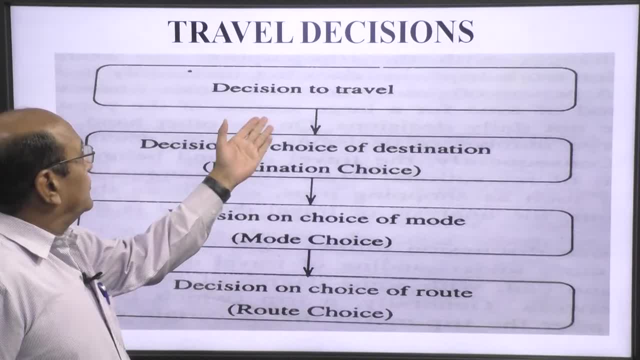 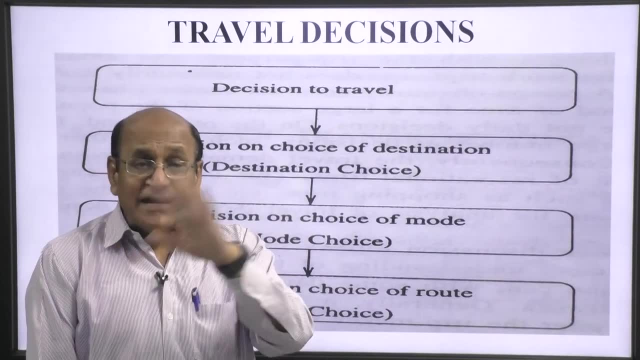 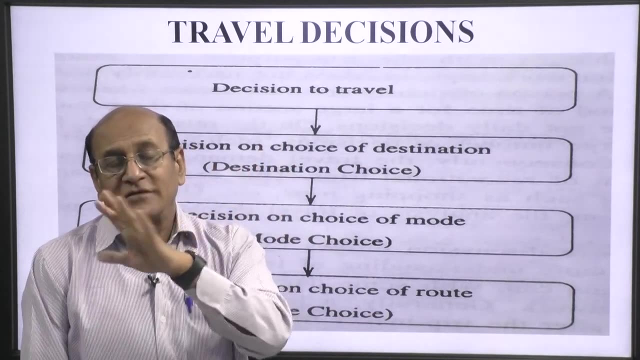 you want to go. suppose one has to purchase a clothes, and there are many destination in Lucknow like Amenabad, Kapurthala, Indranagar, Patrakarpuram, Gomti Nagar, etcetera, etcetera. 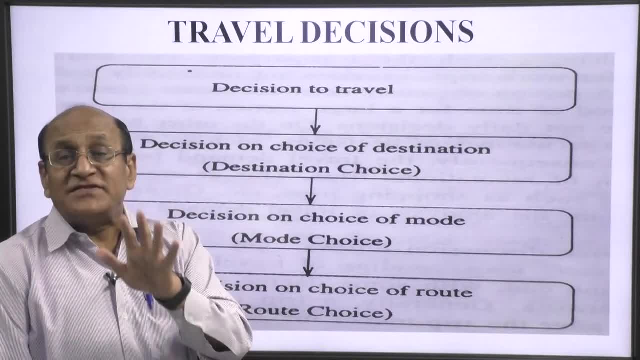 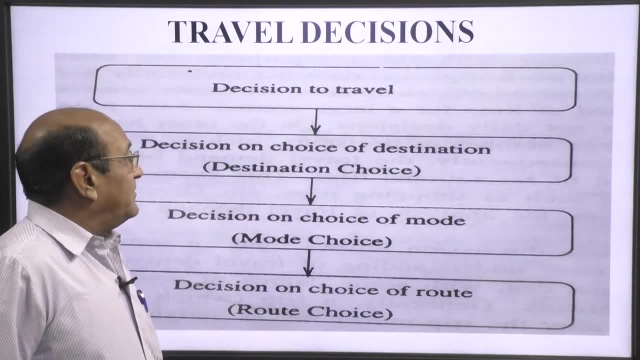 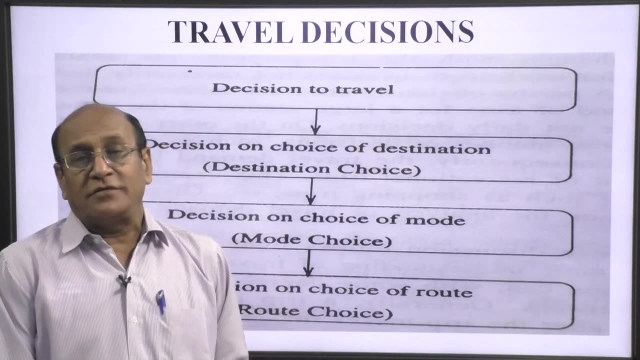 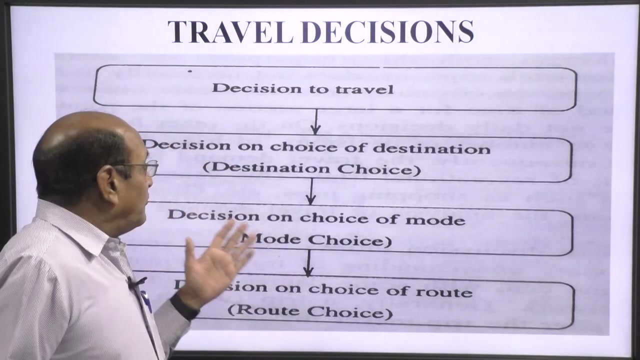 So here he has to purchase a cloth. So he has taken decision to travel. The second step is decision on choice of destination, because there are a number of destination in Lucknow, Places from where he can buy clothes, So he will have to take decision which place. 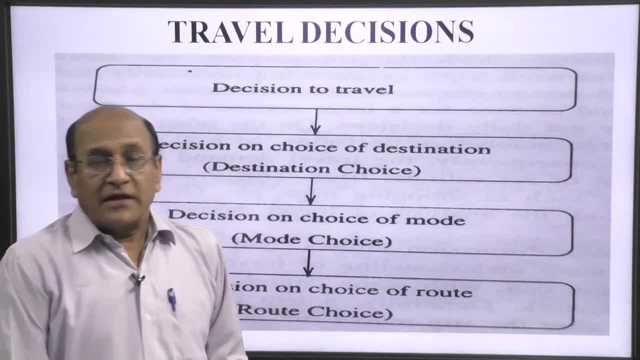 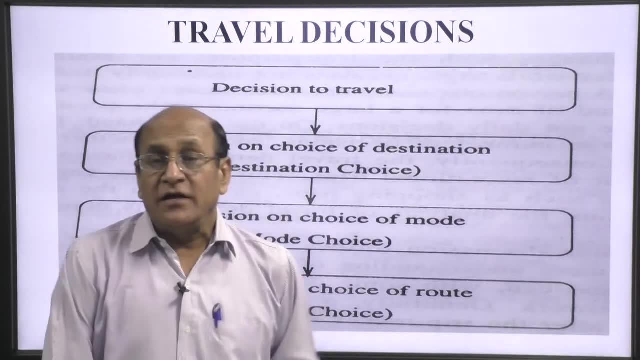 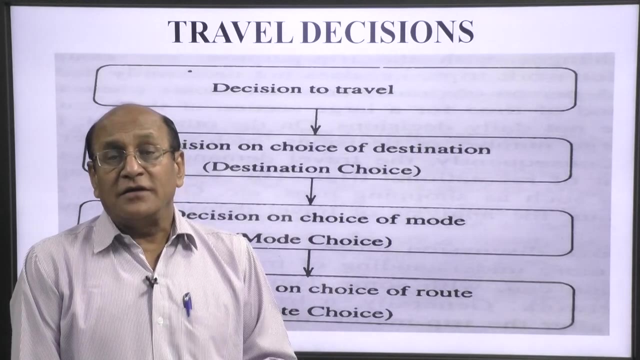 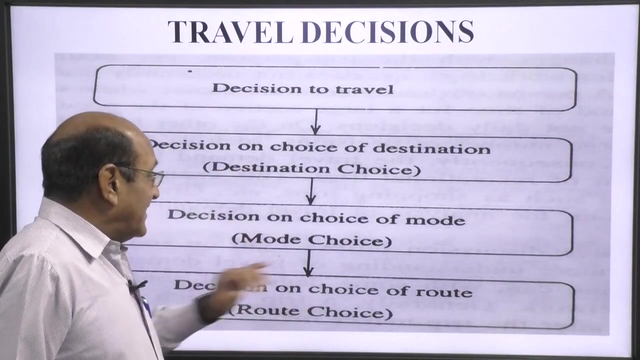 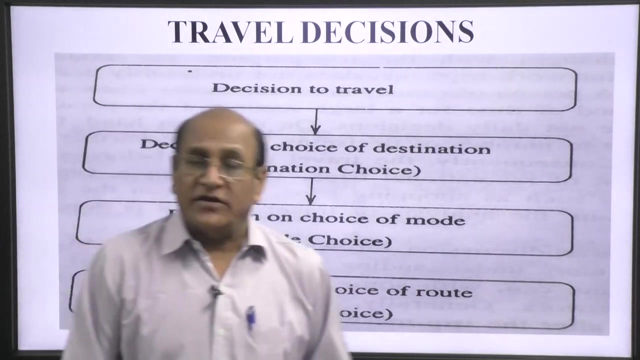 he is choosing for purchasing, Then the next, after this, the next is decision of choice of mode, which mode he will go for that particular place: by two wheeler, four wheeler, hired vehicles, share vehicles, etcetera, And after that then he will decide with which route he will go for purchasing their. 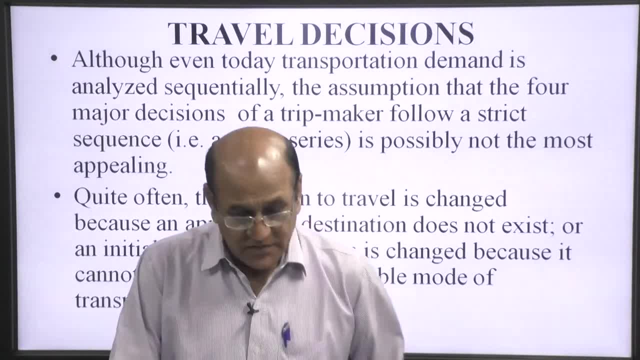 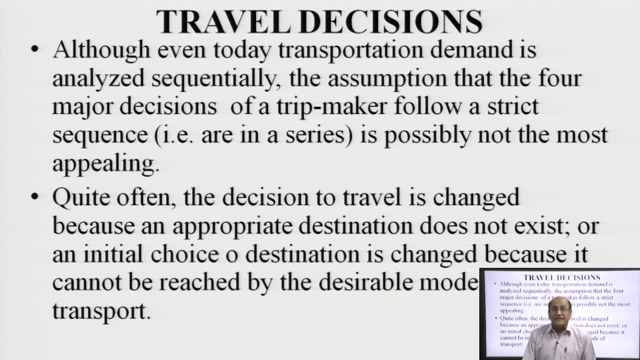 clothes. Although even today transportation demand is analyzed sequentially, The assumption that the four major decision of a trip maker follow a strict sequence Or in the city, is possibly not the most appealing. Quite often the decision to travel is a changed because of appropriate destination does not exist, or any initial choice of destination. 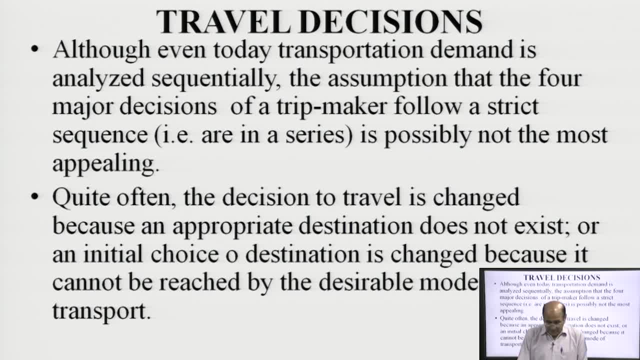 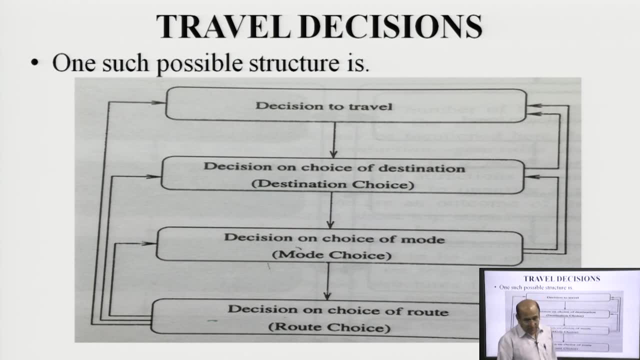 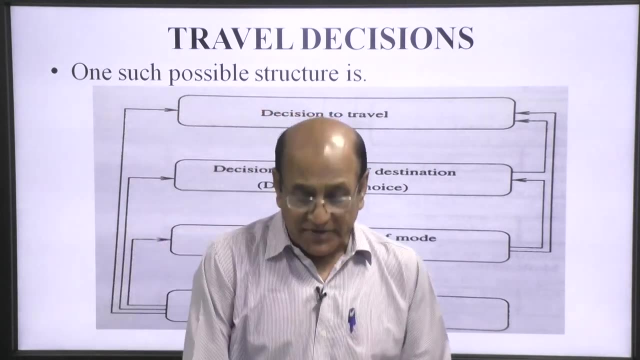 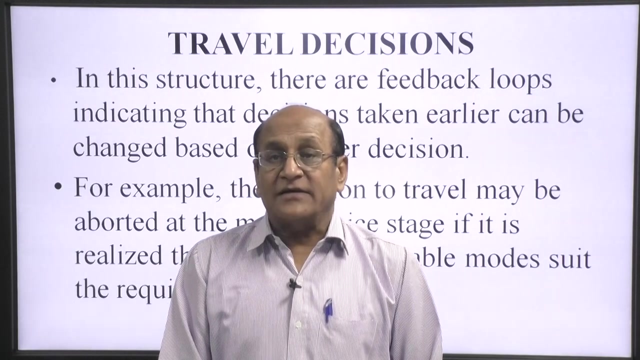 is changed because it cannot be reached by desirable mode of transport, So it is not the most appealing, So this may be changed. So travel decision. again, we have a same diagram. This is the structure of sequential demand. In this structure there are feedback loops indicating that the decision taken earlier. 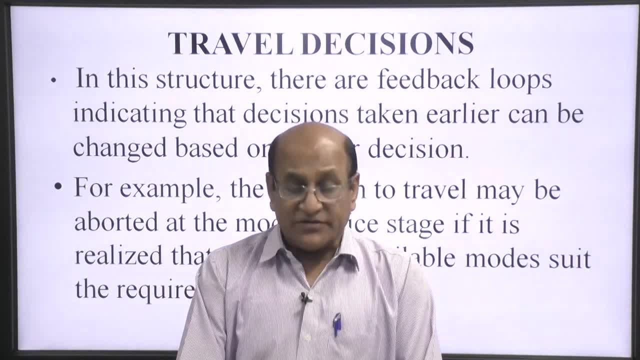 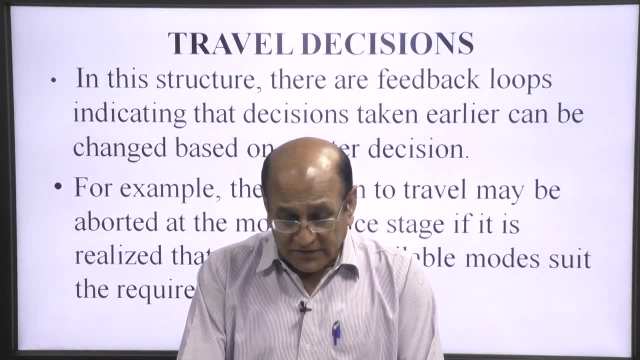 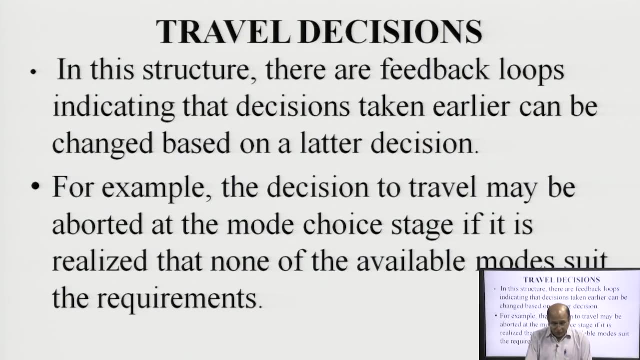 can be changed. So this is the same structure. So in this structure there are feedback can be changed based on later decision. For example, the decision to travel may be aborted at the mode choice stage if it is realized that none of the available modes suit the. 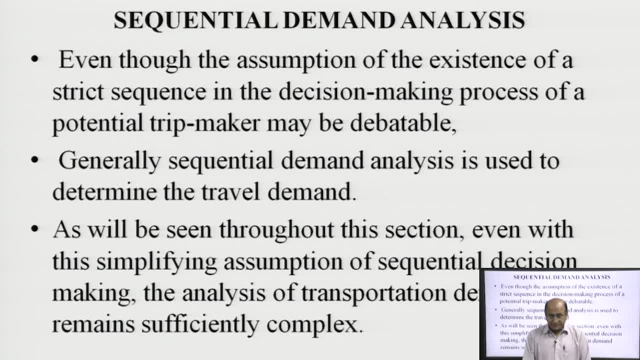 requirements. Then sequential demand analysis. even though the assumption of existence of a strict sequence is decision making process of a potential tip maker may be debatable, Generally, sequential demand analysis is used to determine the travel time I will demand, as will be seen throughout this section, even with this simplifying assumption, 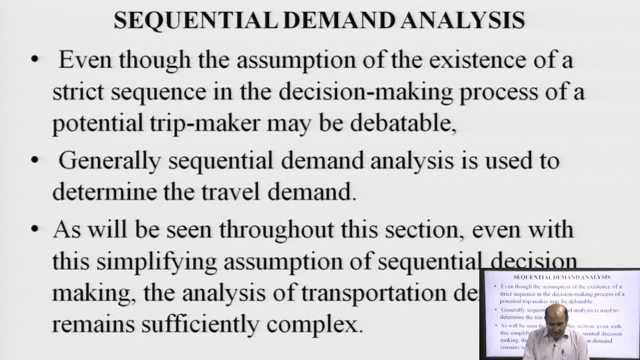 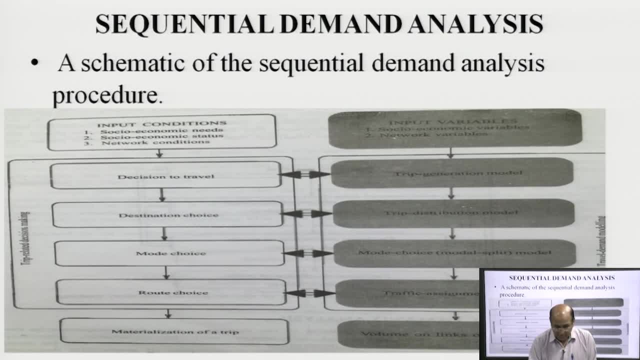 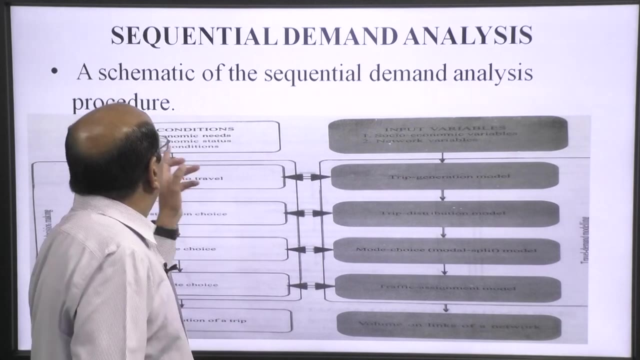 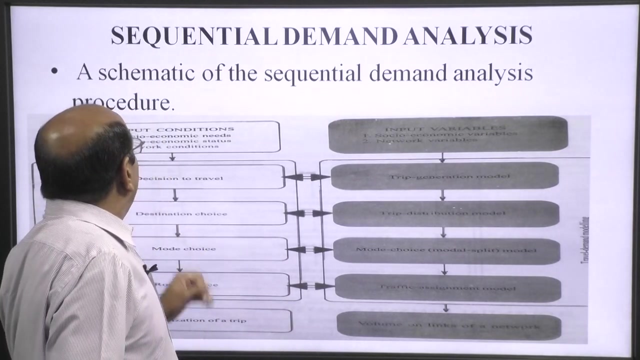 of sequential decision making. the analysis of transportation demand remains sufficiently complex. So here a systematic of sequential demand analysis procedure is given here. These are the inputs. input condition that include socio economic need, first of all, The second, socio economic status, and third, network condition. 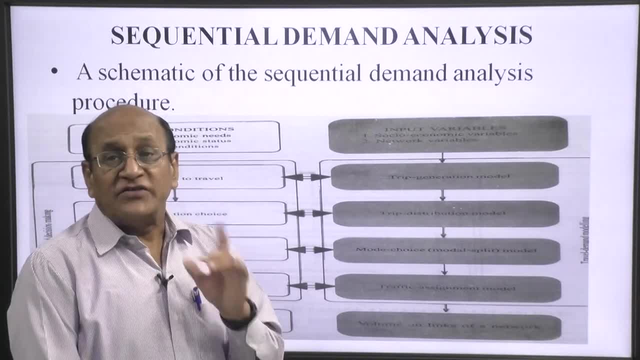 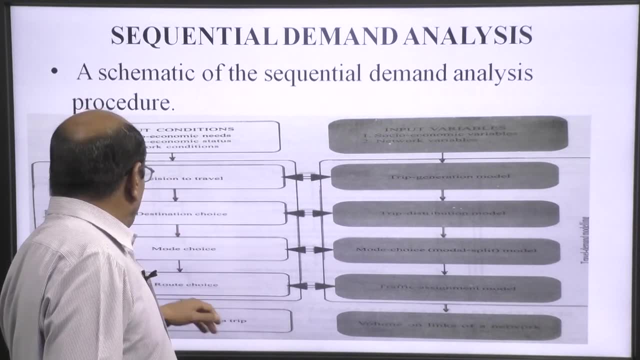 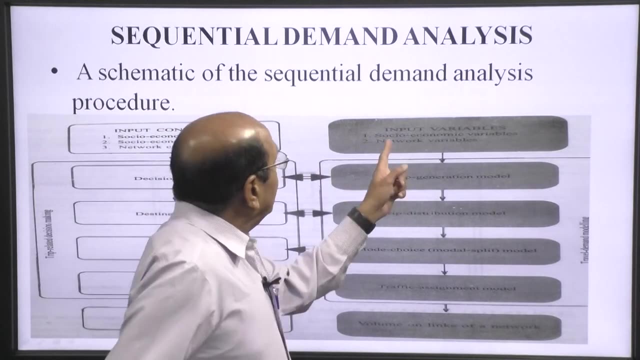 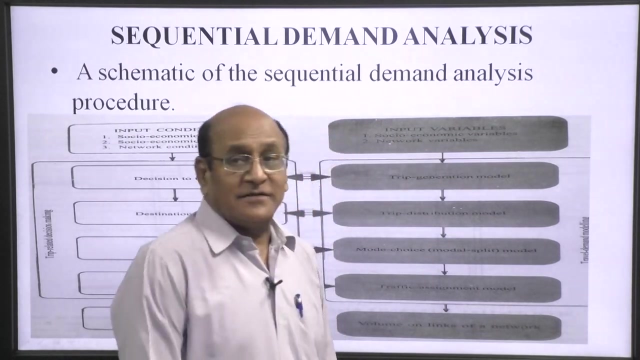 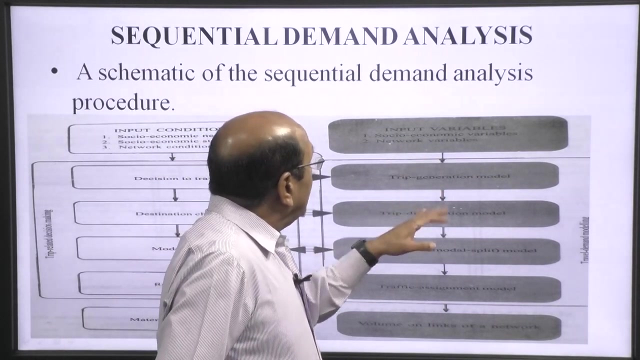 these are the basic input for the sequential demand and these are the decision to travel, choice mode, choice route, choice and materialization of a trip. So we can see here the input variables. What are the variables? Socio-economic variables and network variables. So we can say on the 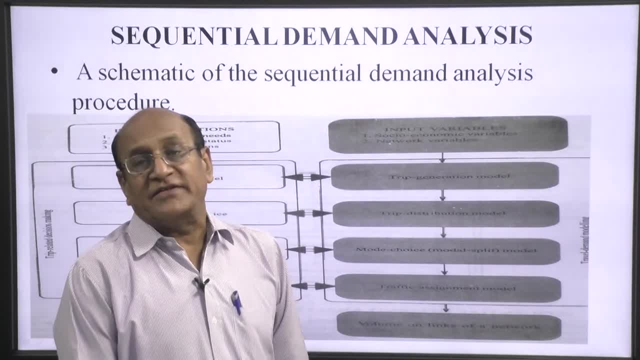 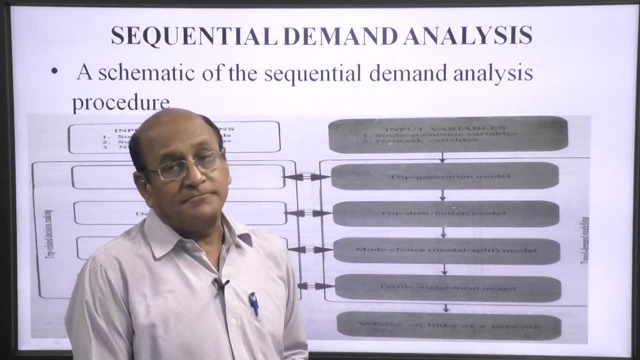 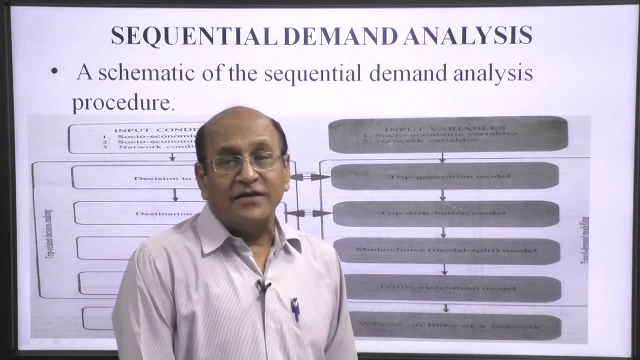 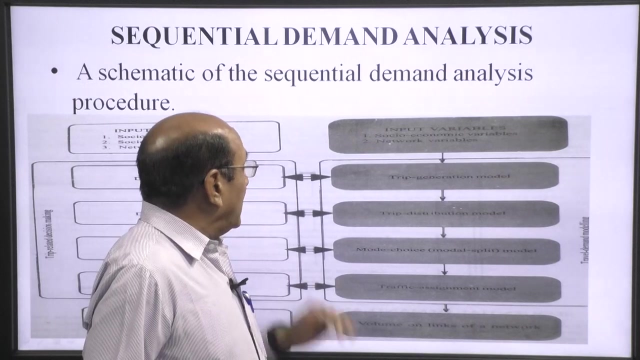 first decision, the trip generation model will come in existence. Then the destination choice, the trip distribution model, will come. The third, mode choice or model split will come in existence. and the fourth, after taking the decision of all above three, then the trip assignment model will come in existence. 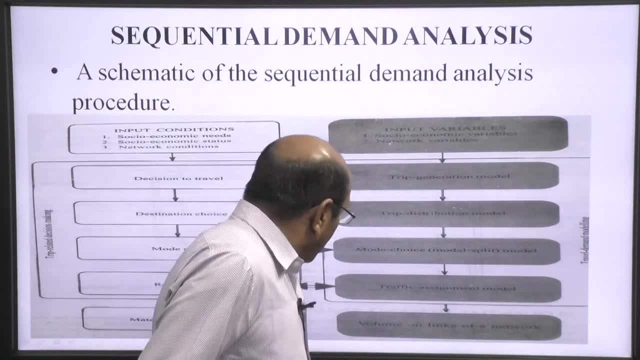 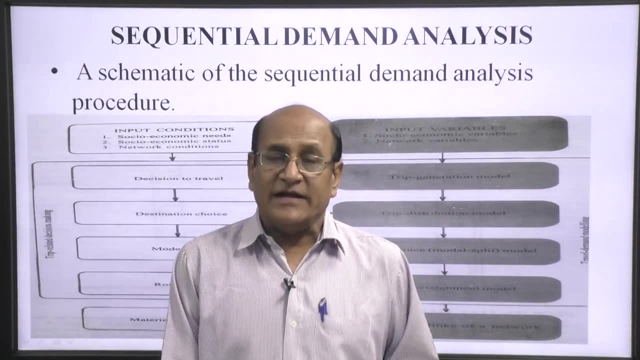 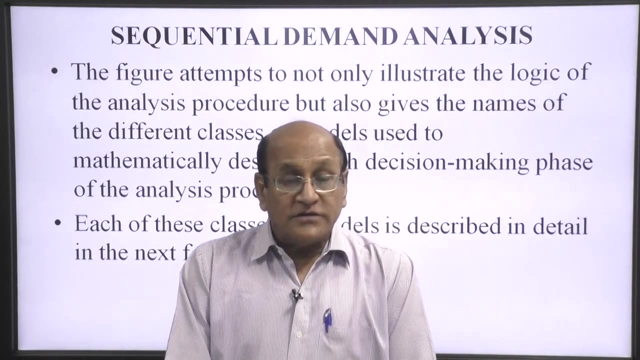 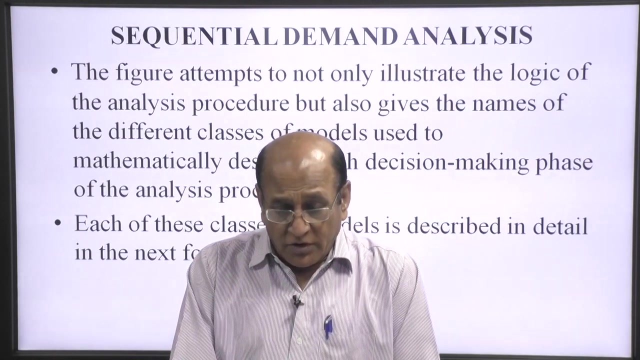 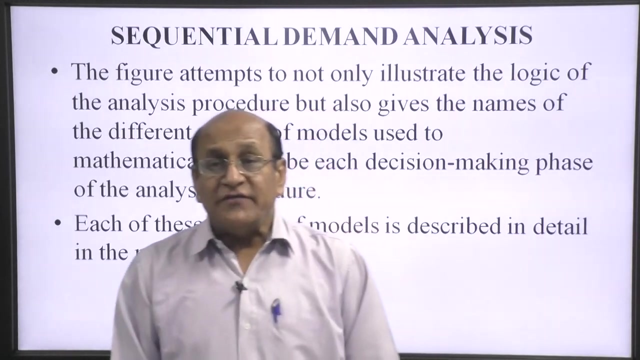 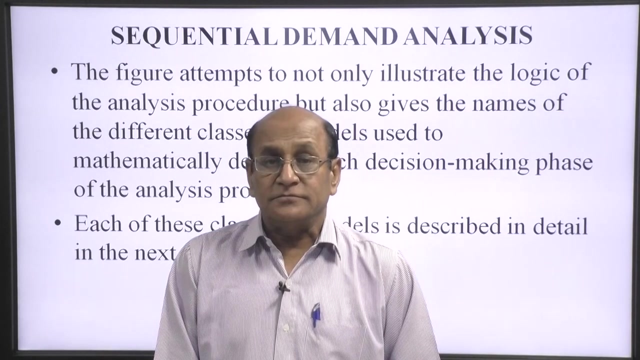 And finally the volume on a link or a network. So this is the sequential demand analysis. on the basis of that that could be done. The sequential demand analysis, the figures attempt to not only illustrate the logic of analysis procedure But also give the name of a different classes of model used to Mathematically describe. 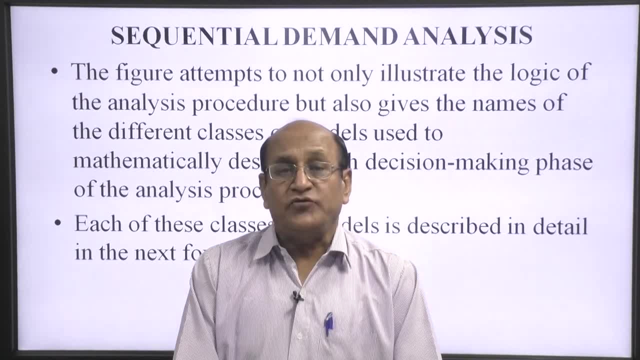 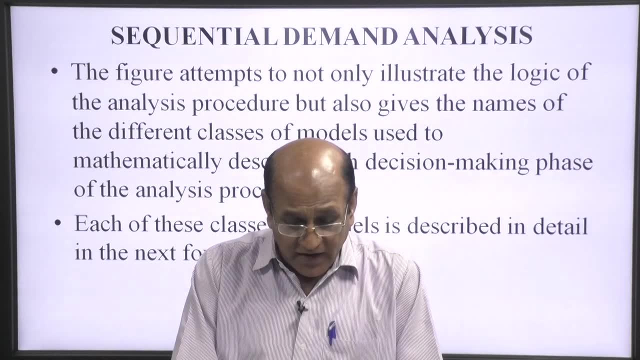 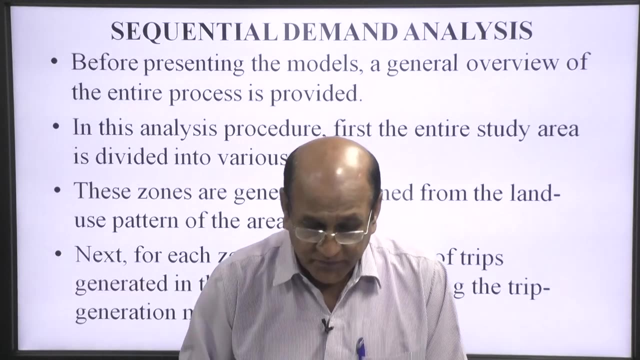 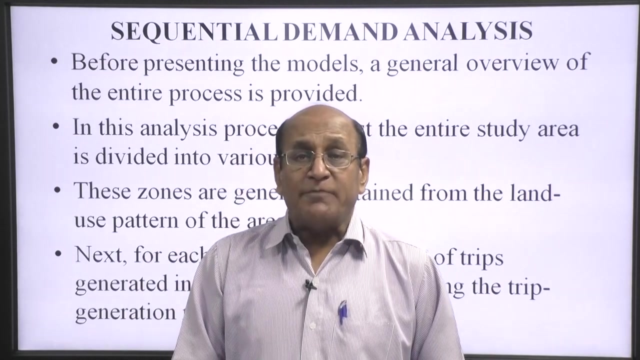 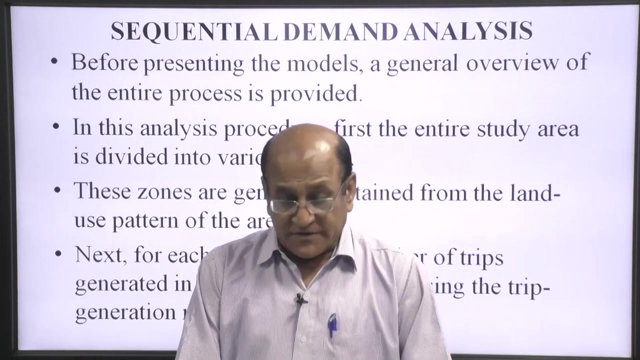 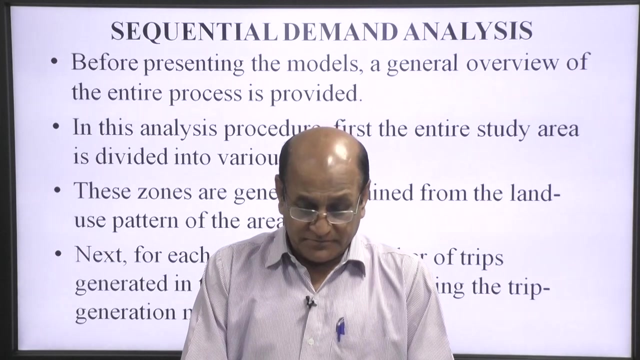 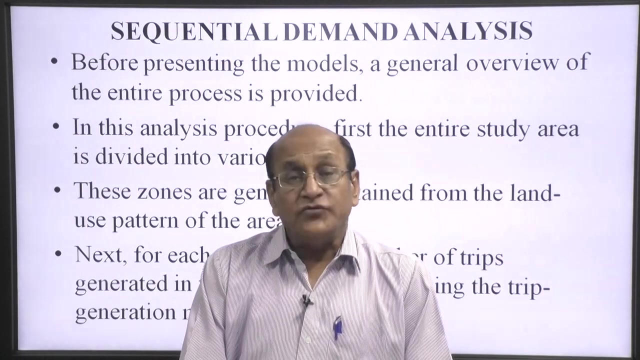 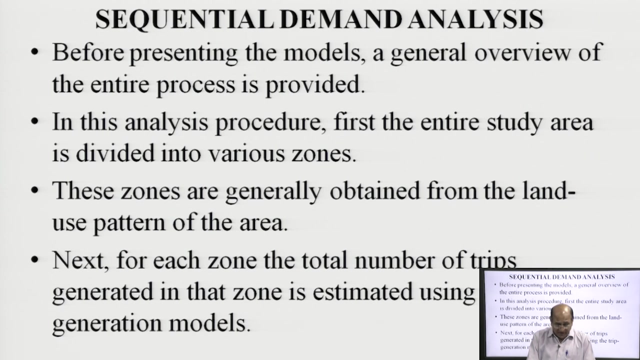 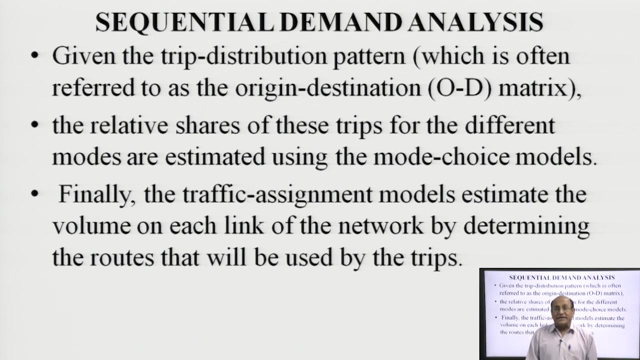 each decision making phase of the analysis procedure. Each of these class of model is described in detail in the next four slides. 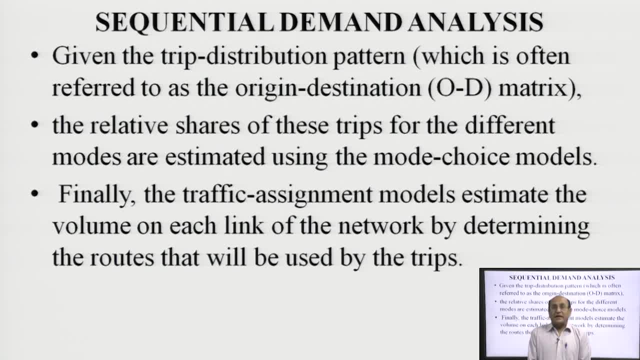 How we will prepare. Suppose certain number of trips are generated in certain zone, So these trips are origin of trips Out of these origin generated. then the trips are divided into different zones- Zone 1,, 2,, 3,, 4,, 5,, 6- and summation of these all trips will be: 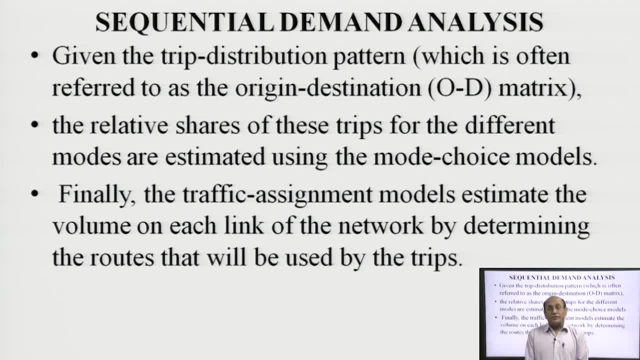 equal to the number of zones, So number of trips generated in zone 1.. Likewise, each zone will create certain trips and that will attract certain trips also. So in this way we can make OD matrix like this way. So 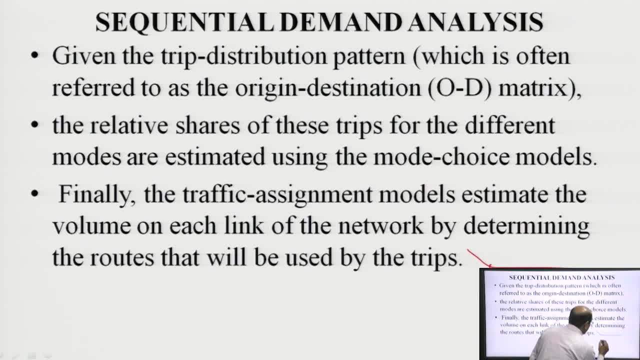 say this is the attraction 1,, 2, 3.. These are the zones 1,, 2, 3.. Number of trip generated in zone 1.. So suppose that is handed. So handed trips could be divided in zone 1 means itself zone. 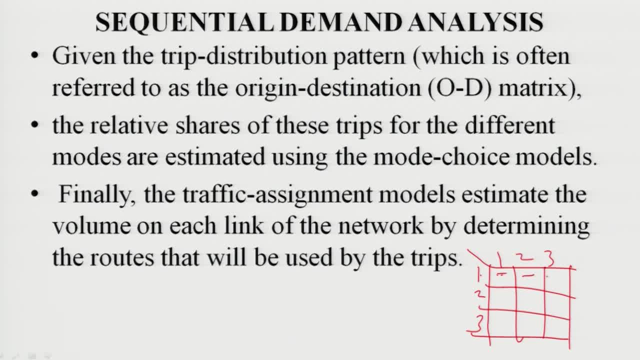 then zone 2, then zone 3.. So this will total will be equal to the total number of trips. total: The trips generated in zone 2 will again distributed or attracted in zone 1, 2 and 3.. The total: 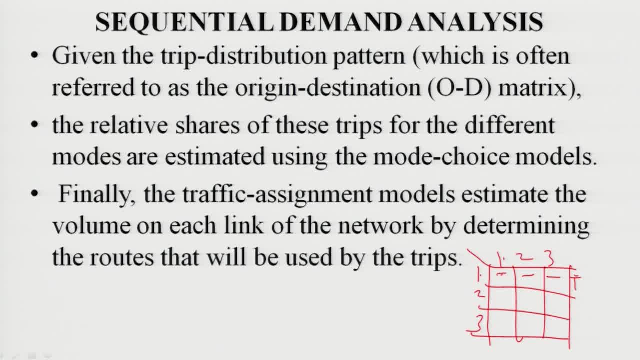 summation of trip in zone 1 and 2 and 3 will be equal to total number of trip generated in zone 2 and same way as in zone 3.. So we can see the total number of trips generated in zone 2.. 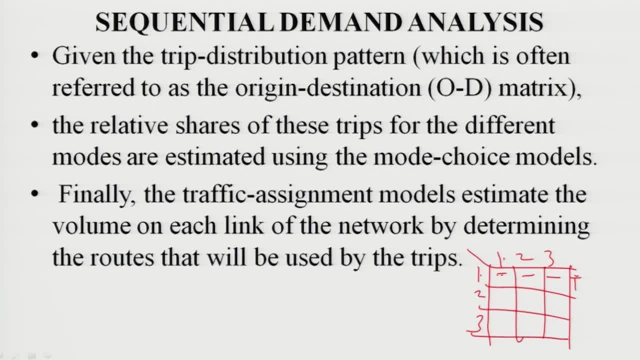 So, in this way, the total number of trip attracted in zone will be summation of this one, this one, this one, and this will be equal to this way. So, again in zone 2, the total number of trip attracted will be summation of trip generated from 1, number of trips.